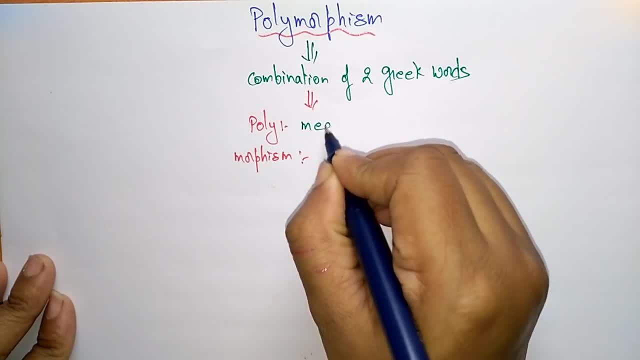 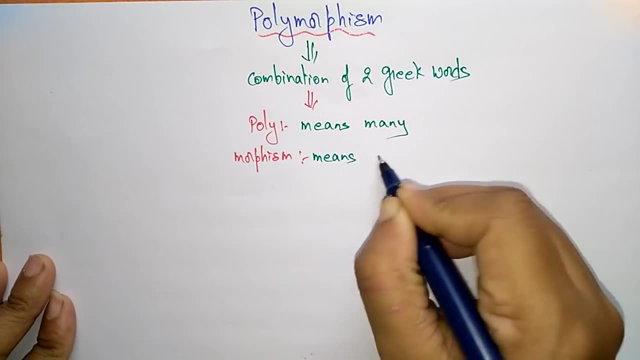 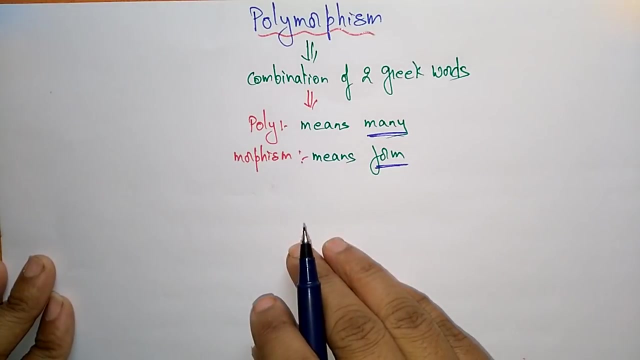 So poly is nothing but means many. Poly means many, Whereas a morphism means form. So what it represent. Polymorphism means many forms. So one thing can be represented in many forms that you call it as a polymorphism. So the functionality of this feature resembles, with its name only. So what its name: Polymorphism, Many forms. 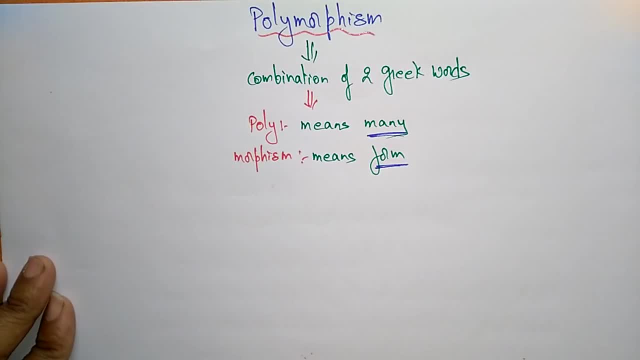 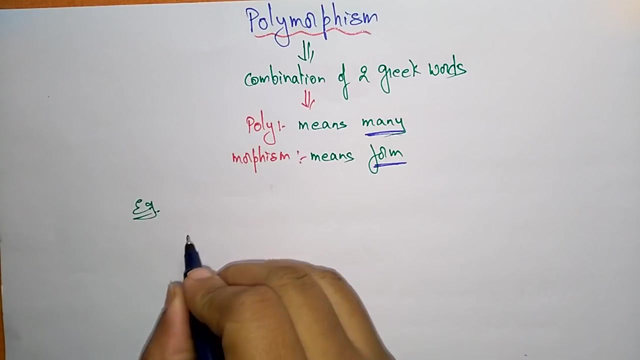 So one thing can be represented in many forms. Okay, So let us see one example to explain this polymorphism. Suppose suppose you are the person, So you are a person. Suppose if you take a person A person, So this person means. suppose a person is yourself only. 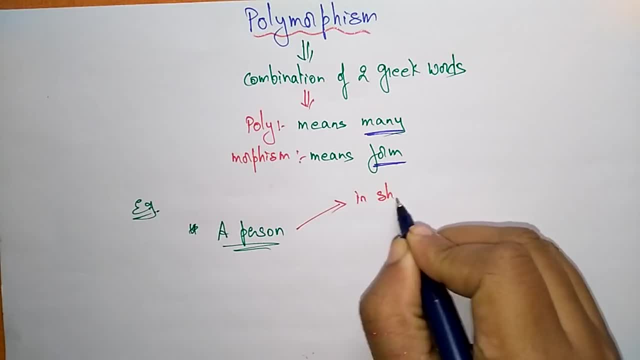 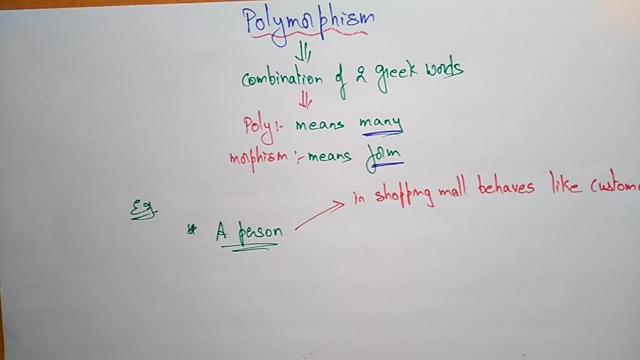 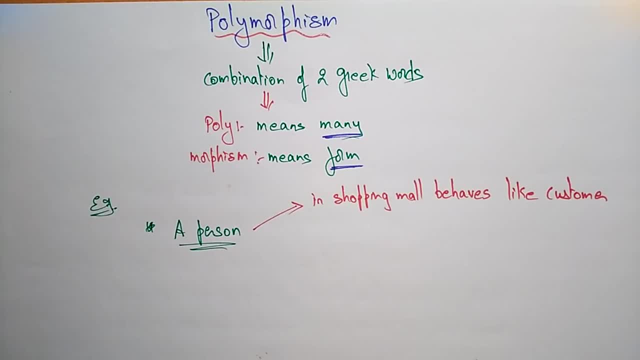 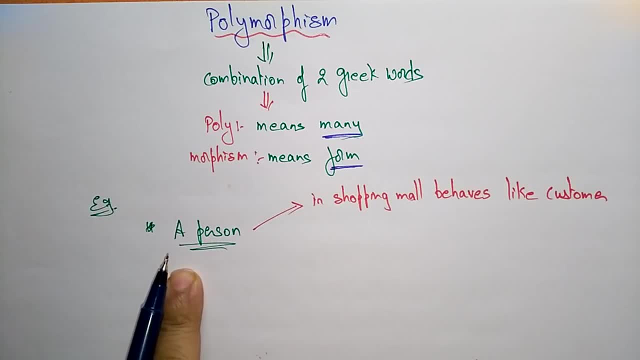 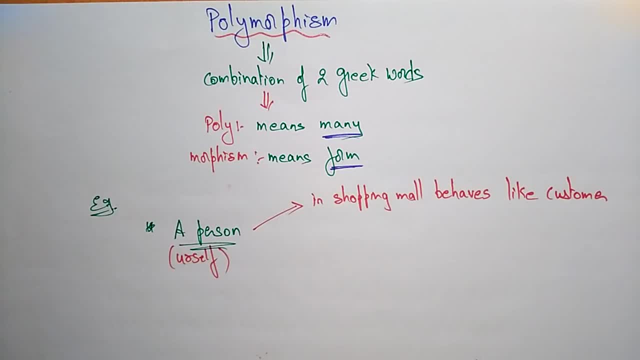 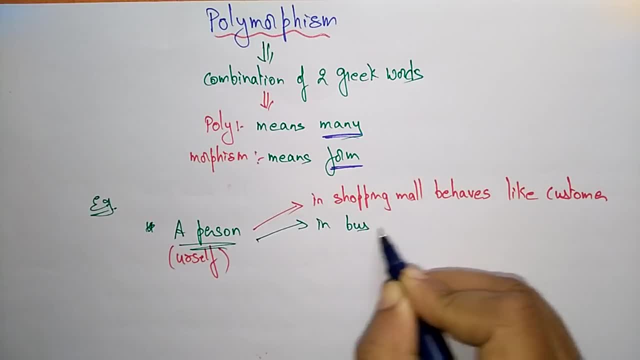 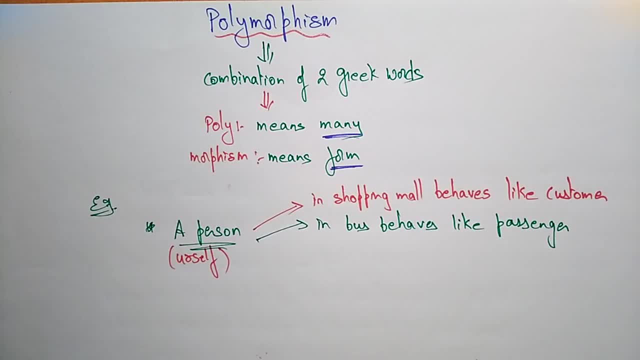 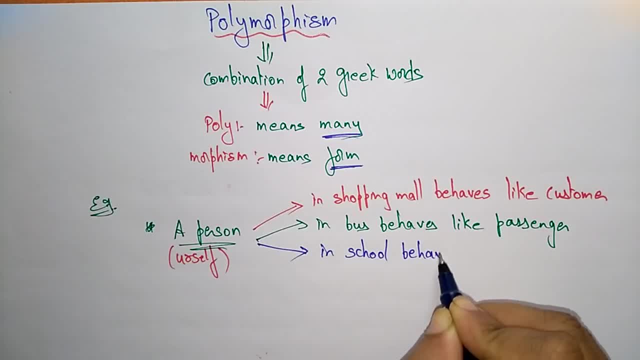 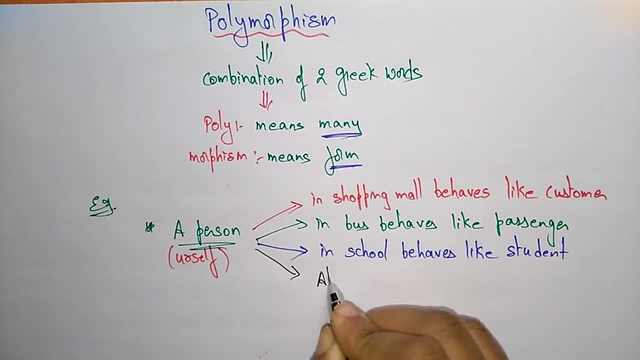 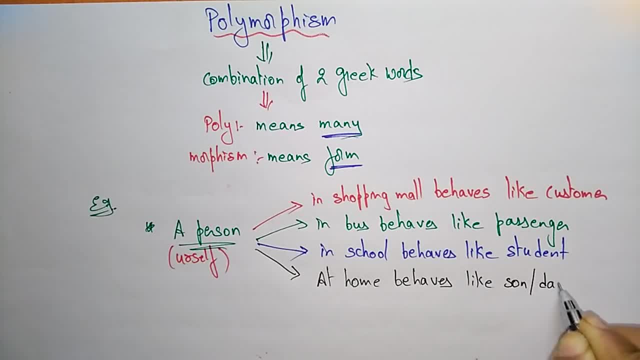 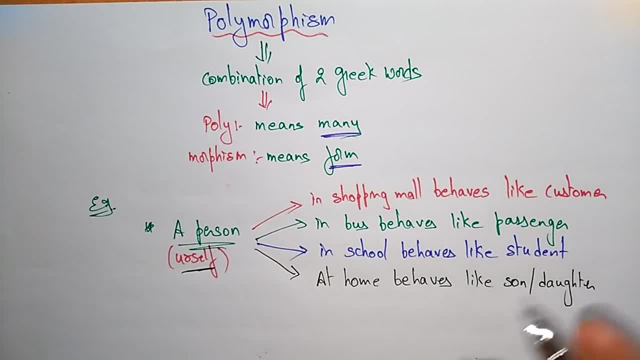 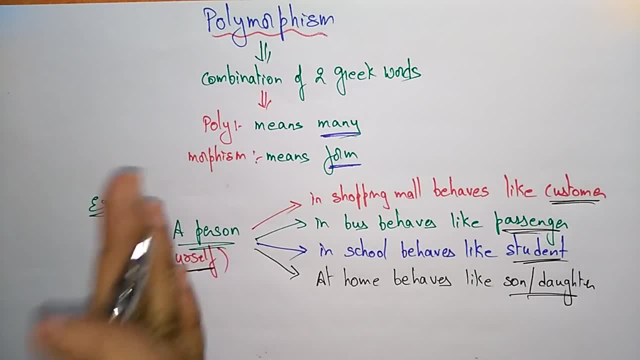 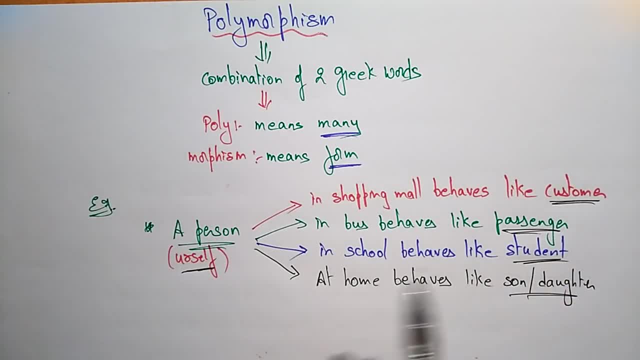 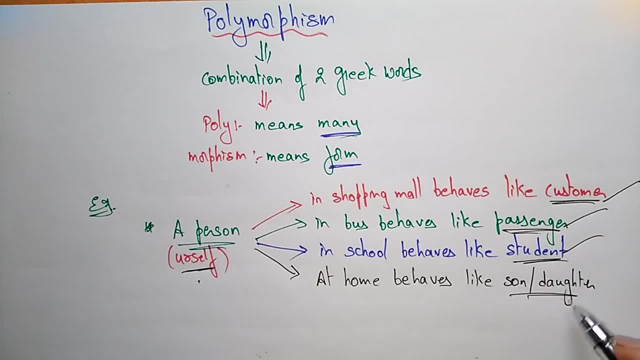 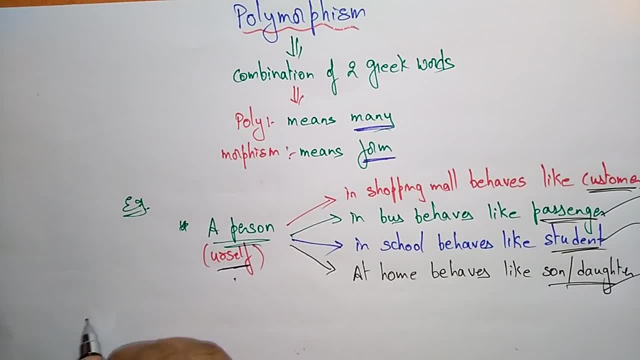 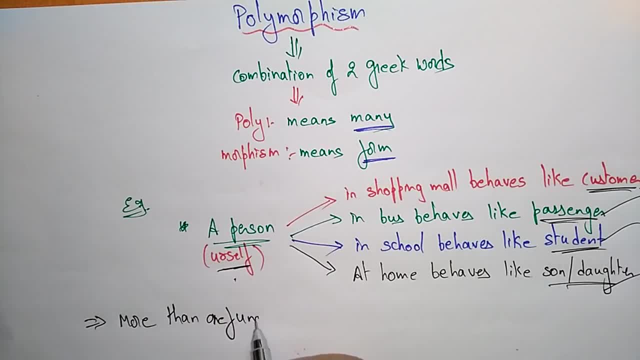 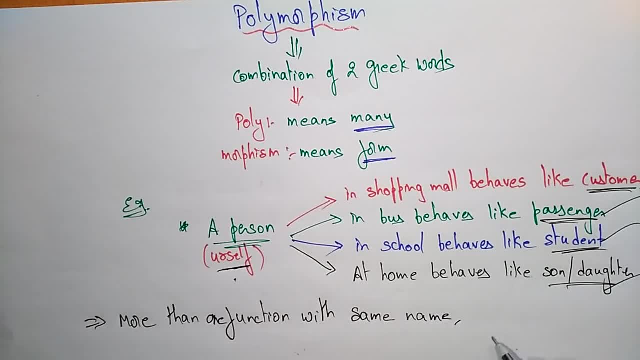 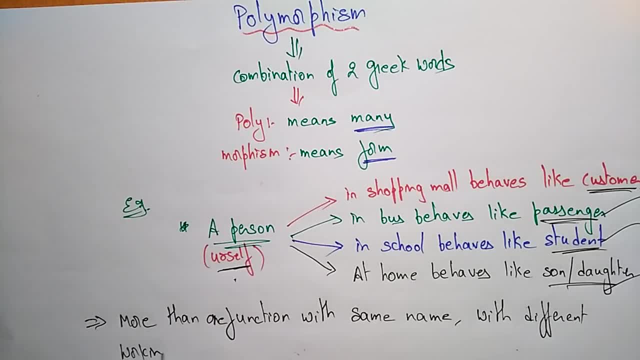 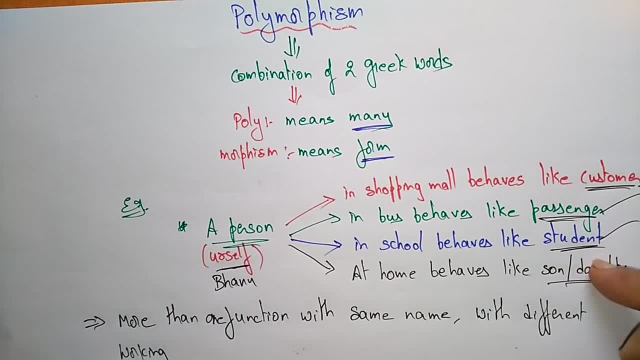 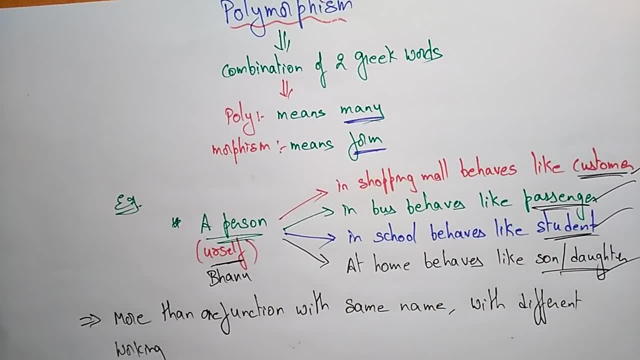 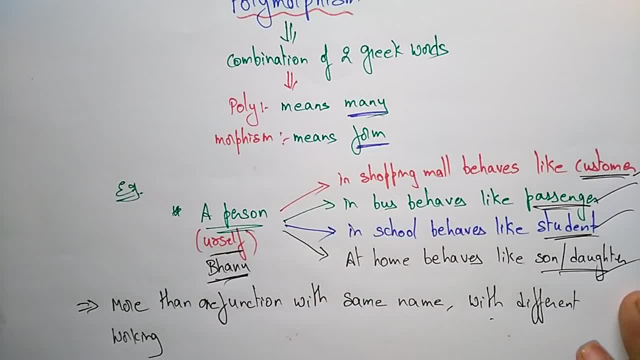 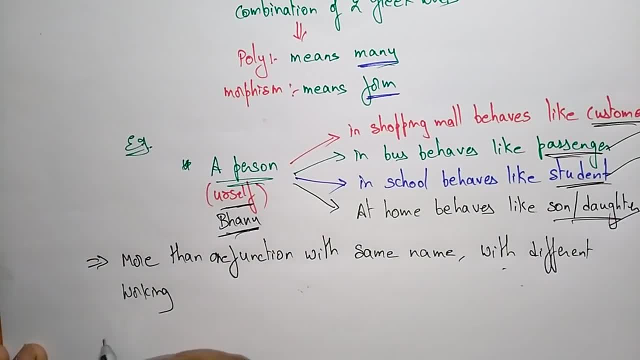 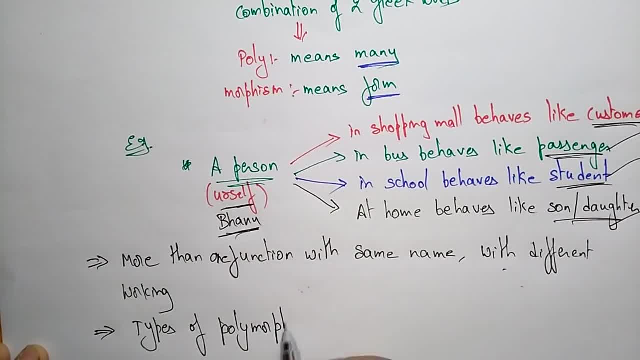 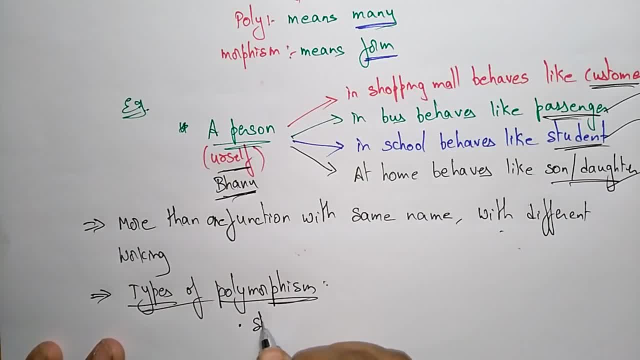 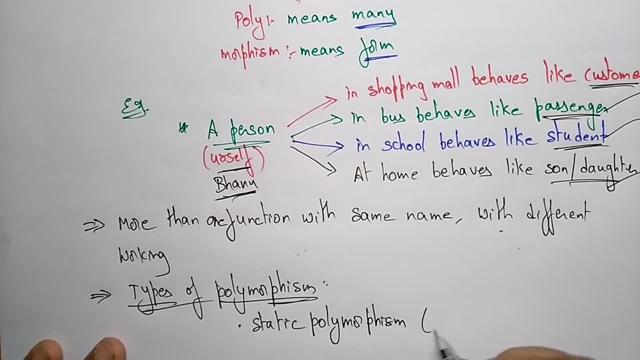 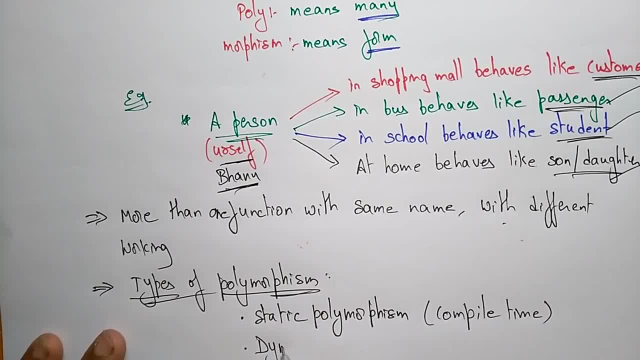 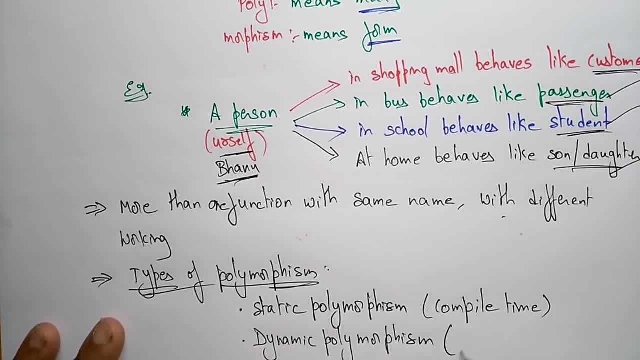 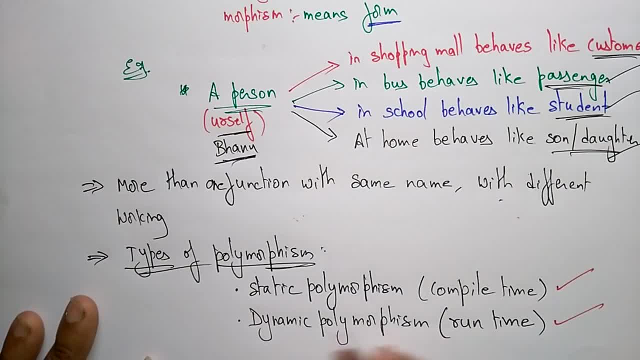 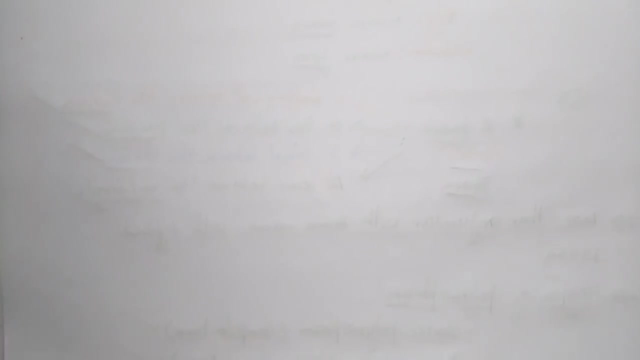 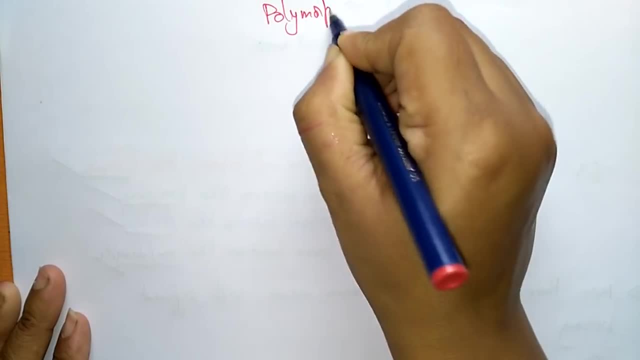 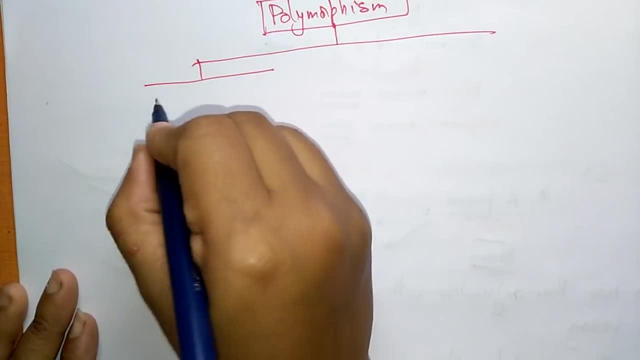 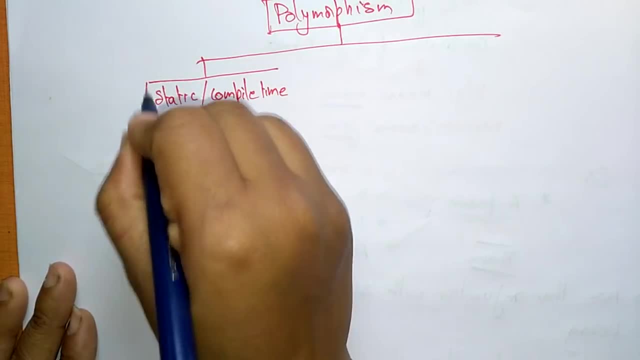 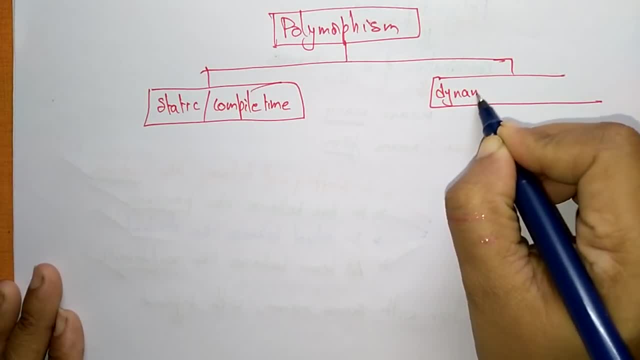 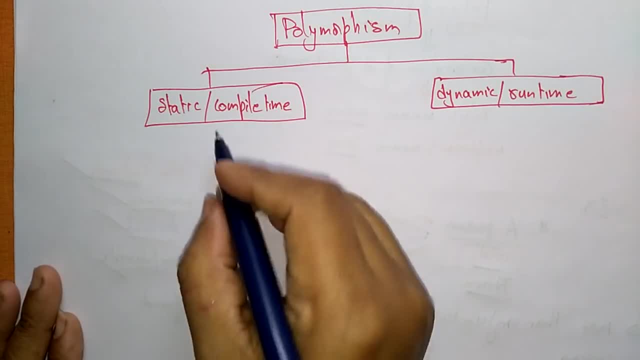 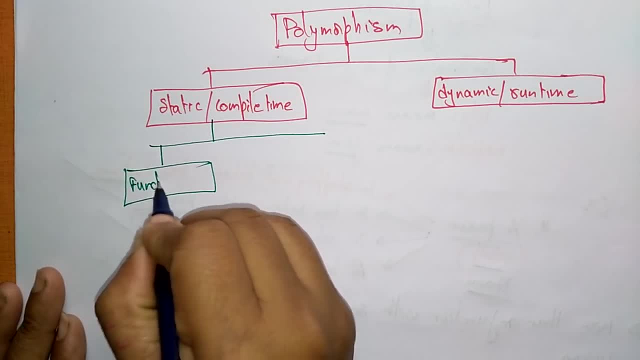 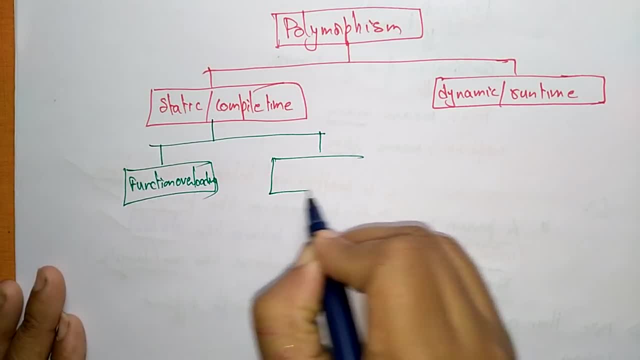 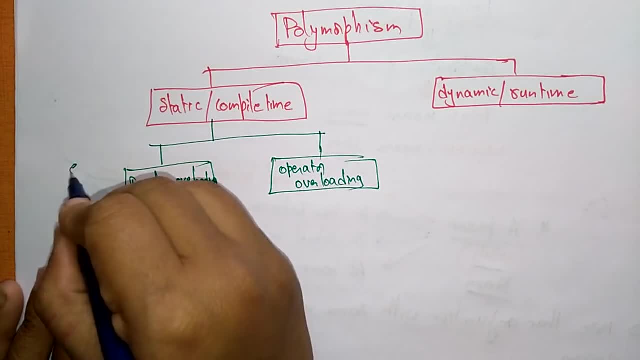 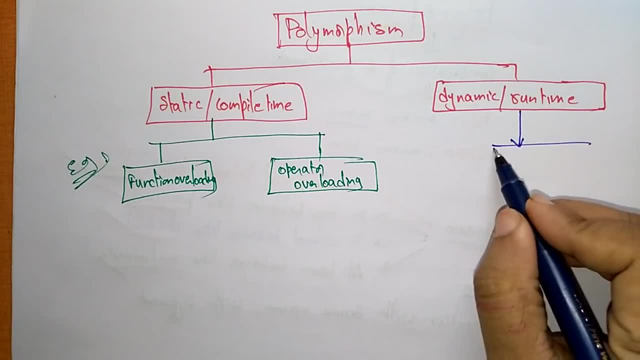 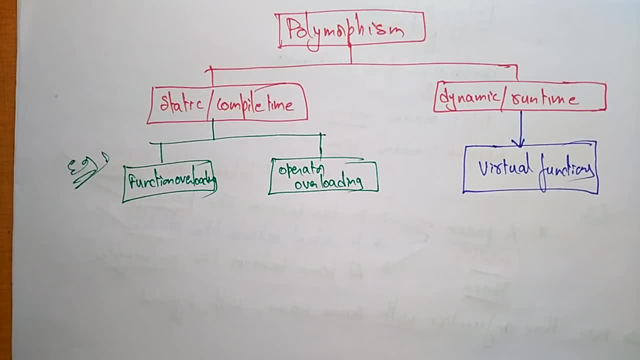 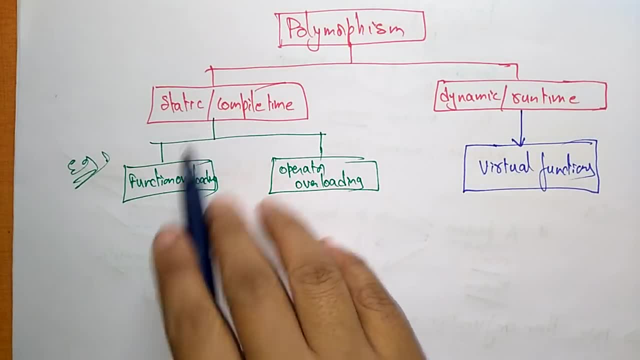 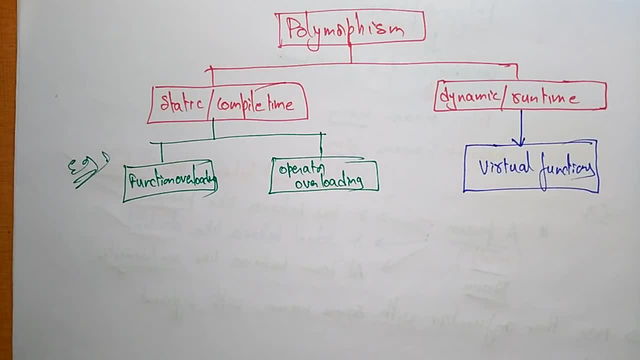 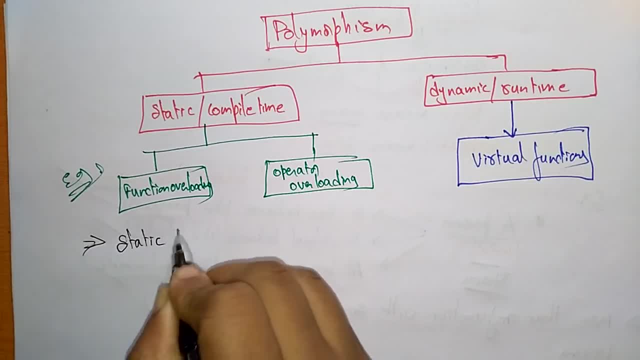 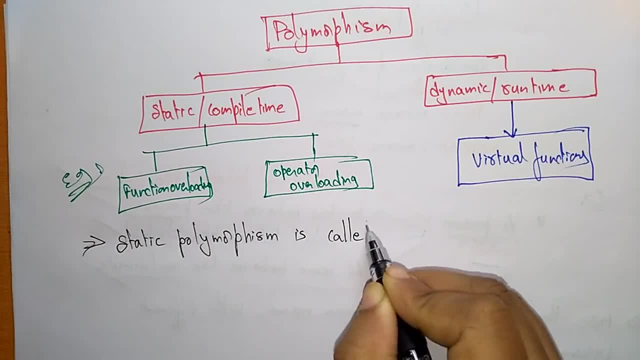 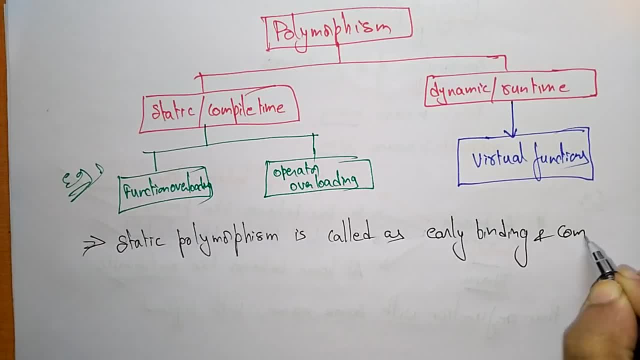 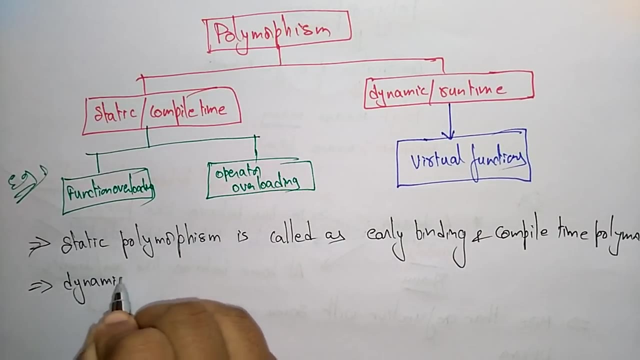 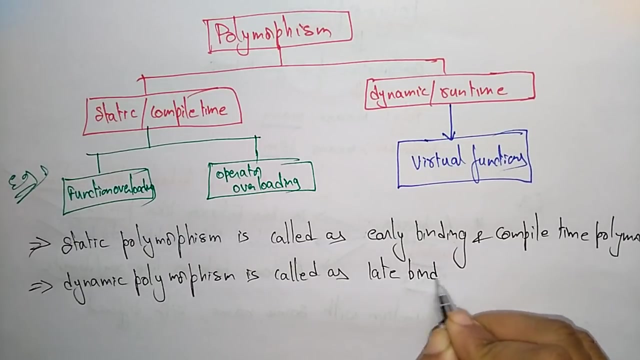 Suppose you are in a shopping mall, You behaves like a customer. Suppose you are in a shopping mall, You behaves like a customer. time polymorphism, Okay, And coming to dynamic, dynamic polymorphism is also called as late binding. So static is early binding, dynamic is late binding and runtime polymorphism. So the main 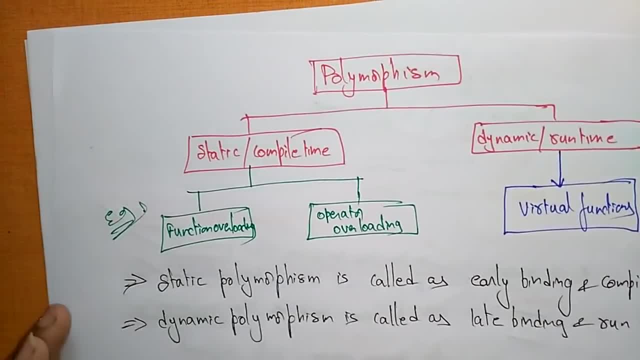 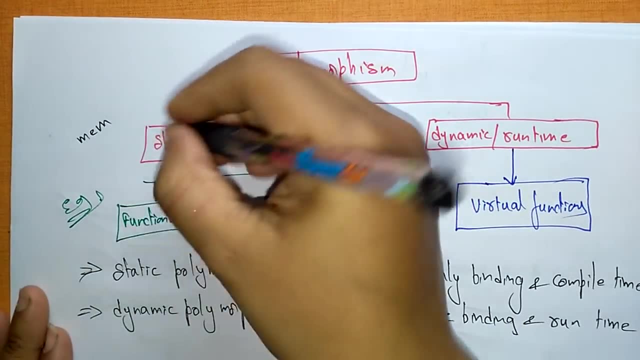 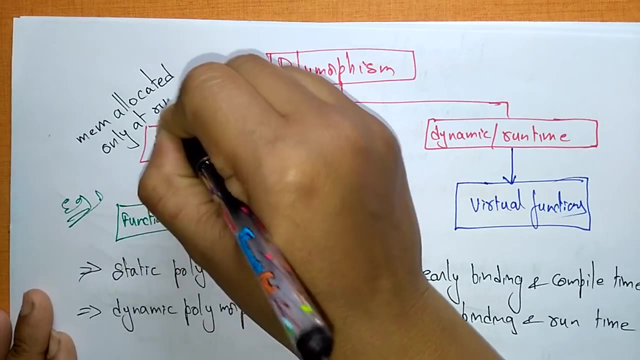 difference between static and dynamic means here. the static means the memory allocated only at compile time. So when you are using the static, it means memory will be allocated only at runtime. That's why we call it as a runtime polymorphism. The another name for static is: 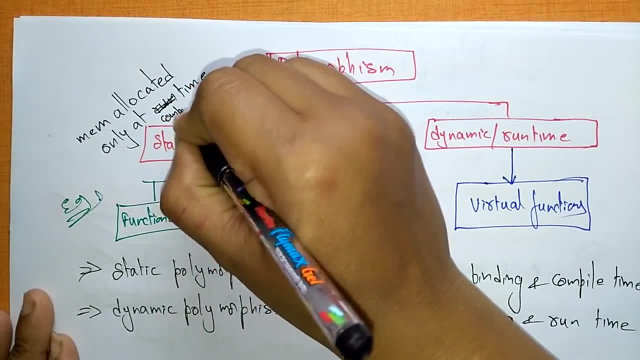 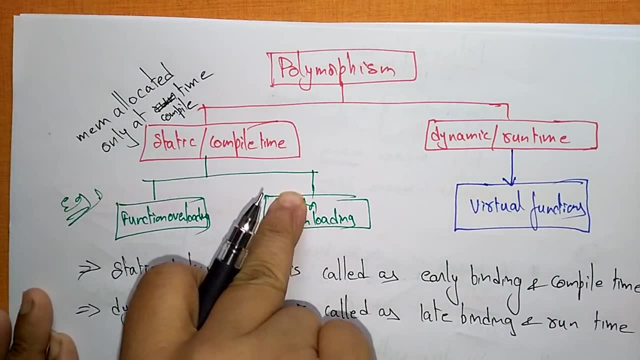 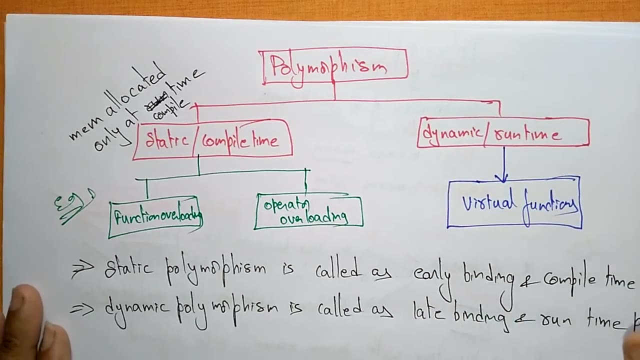 sorry, compile time, I'm sorry, compile time. So this is static. So why we are calling it as a compile time? Because the memory will be allocated only at compile time. That's why we call it as a compile time. polymorphism: The another name for static polymorphism is compile time, Because it 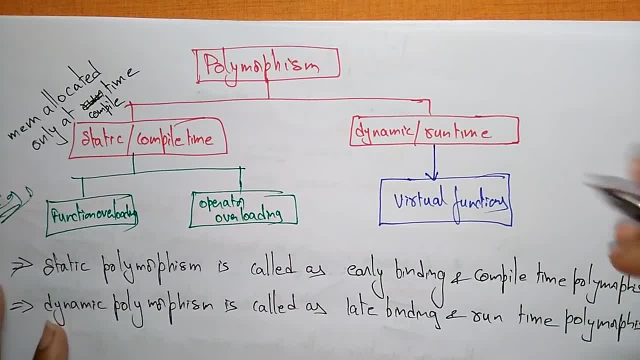 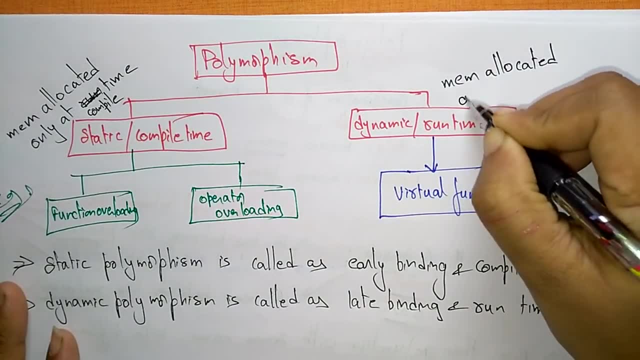 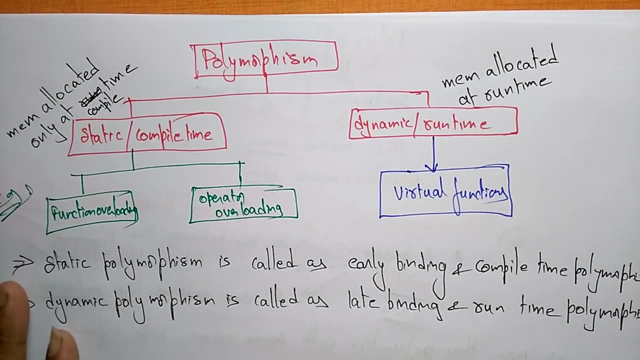 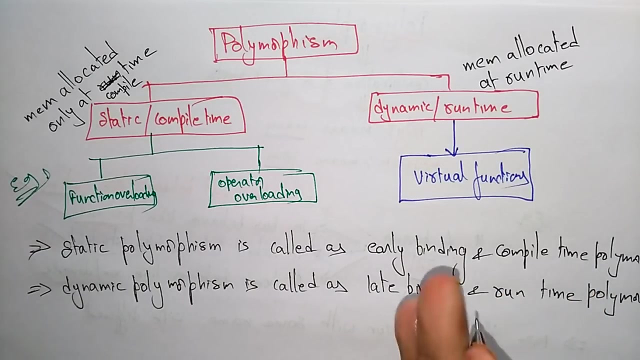 is allocated the memory only at compile time, Whereas dynamic means memory allocated at runtime. So at the runtime only the memory will be allocated That you call it as a dynamic polymorphism. Okay, So this is the introduction of the polymorphism. So in this I explained the definition of the.